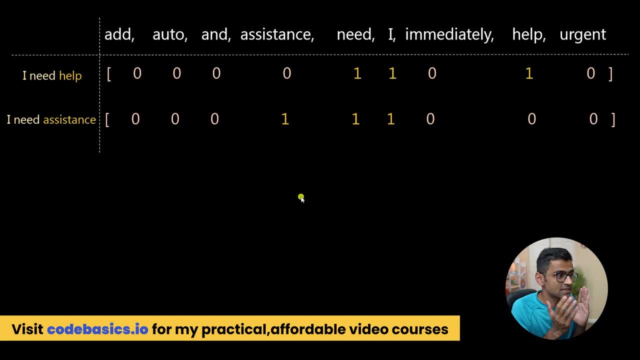 vector representation should be similar. You expect that the representation should be similar, But since these are TF-IDF and bag of words are count based methods, the vector representation might not be similar. Here you can see, see, there is one here, zero here, one here, zero here. 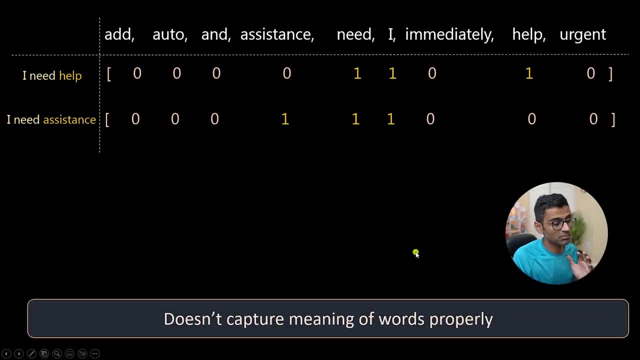 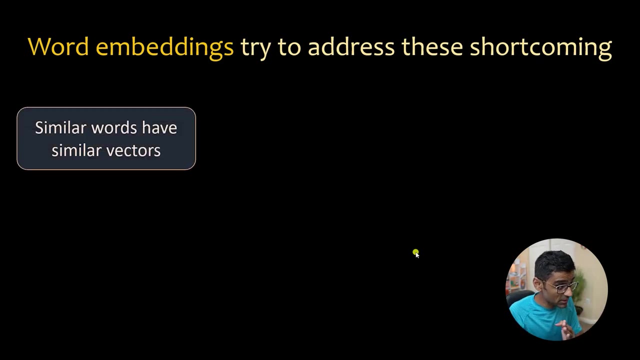 So these techniques do not capture the meaning of the words properly. You expect that if you have two sentences which are similar, their vectors should be very similar. Word embedding tries to address both of these shortcomings. First, similar words will have similar vectors. similar words or even sentences. For example, good and great, these are two similar words. 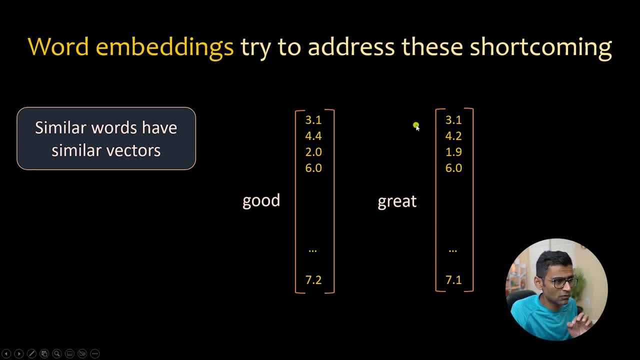 When you will use word embedding, you will notice that their vector will be very similar, See 3.1, 3.1, 4.4, 4.2.. There will be slight differences, but mostly they will be similar. They will also. 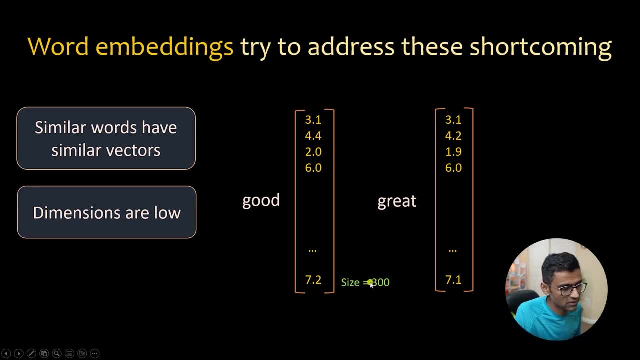 be lower in dimension, which means the size of this vector will be 300.. 300 is one of the popular vector sizes. in word embeddings It could be 50 size, 100 size, etc. But it won't be like 100,000, because your vocabulary size is 100,000.. 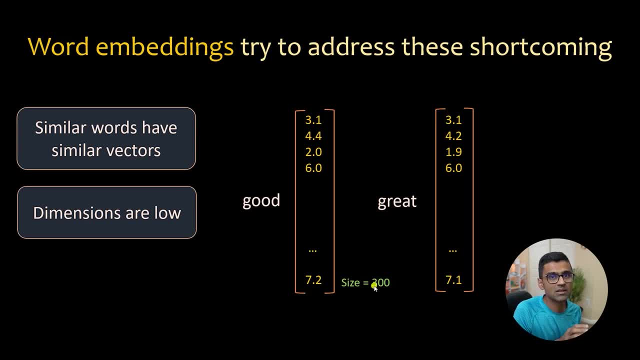 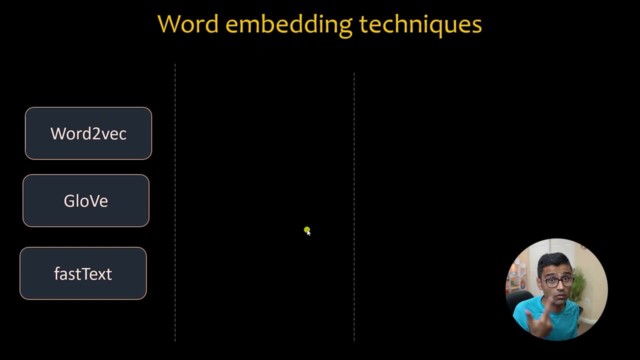 And these representations are dense representation, meaning you won't notice too many zeros, as opposed to the previous techniques where most of the values in the vectors were zero. Now there are various word embedding techniques, such as Word2Vec, Glow, FastText. These are the techniques which are 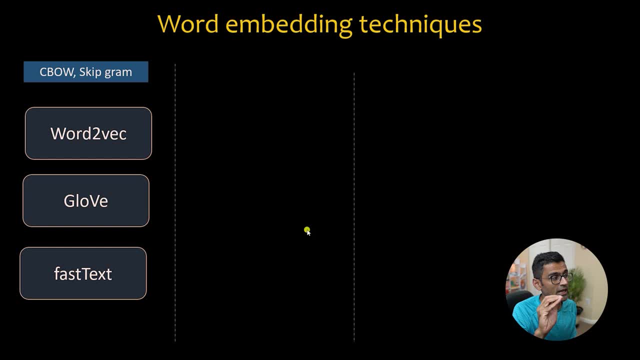 built on different approaches, and the common technique that we use to build these word embedding, which is Word2Vec, Glow and FastText, is using continuous bag of words and skip gram. Now this might be jargon, so just hold on. I will go over that in detail a little later. 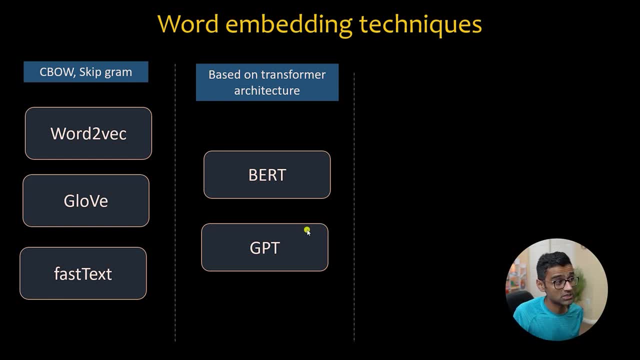 Then there are techniques such as BERT and GPT, which are transformer-based embedding techniques. These are the latest advancements in NLP. When you do Google search, it is using BERT, So you might have heard all these jargons. So I am just going to go over these jargons in brief and in the later videos. 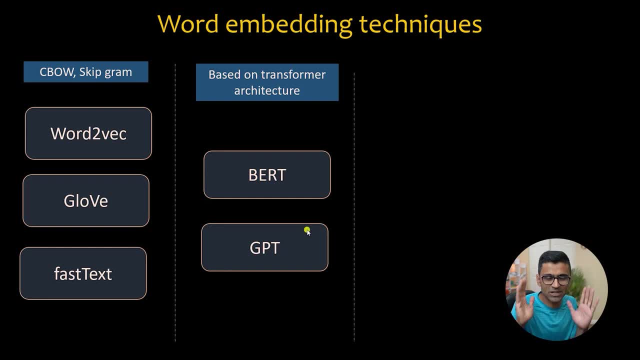 we will go over them one by one, So don't worry if you are confused right now. just don't worry. Just remember that these are various word embedding techniques. There is a technique called the DIAMO, Which is based on LSTM. Now, what do these techniques do? 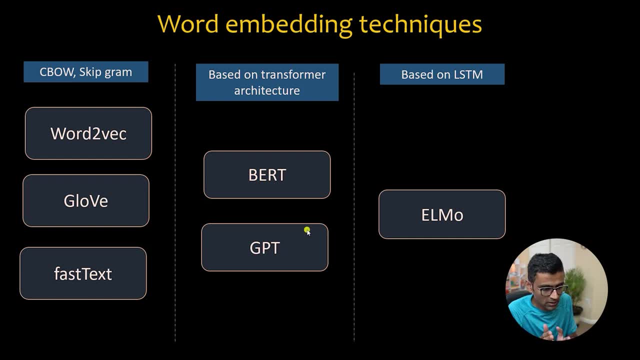 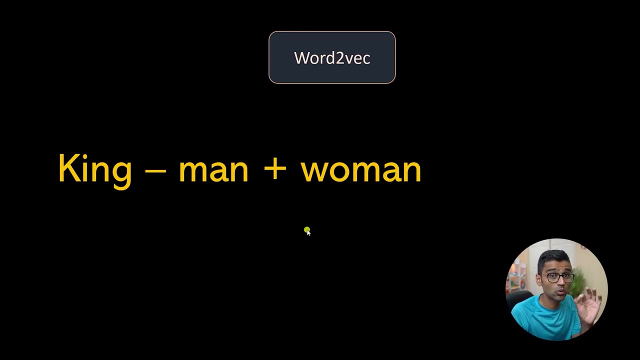 They convert a word or a sentence into a vector representation so that it can capture the meaning of that word properly. Not only that, you can do arithmetic with the words. Word2VEC has this famous example that you can do arithmetic. You know how you do arithmetic with numbers. 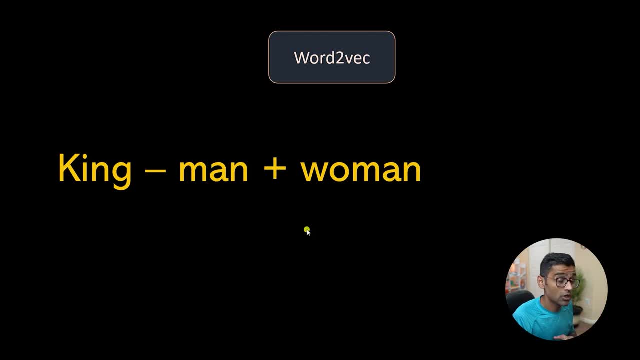 Let's say: two plus three is equal to five, minus one is equal to four. You can do similar things with the tax, and that's mind-boggling, right see king. king has all these attributes: authority, king is rich, it has power. but if you remove the element of men from that and add woman, 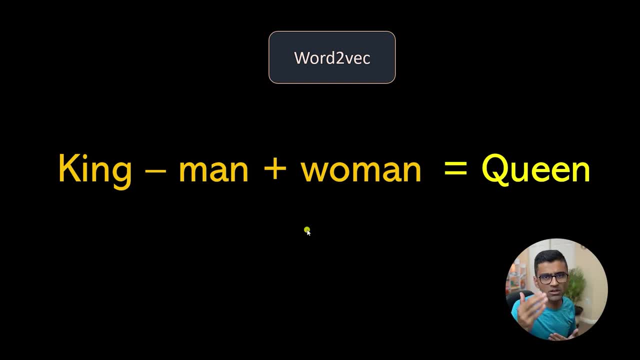 it becomes queen. correct. queen also has power, authority, lot of money, but the gender is different. so you subtract the gender, add a new gender. now you get queen. we'll look all of this in detail. we'll look into this in in the detail, uh, during the code. but for word2vec, i have already. 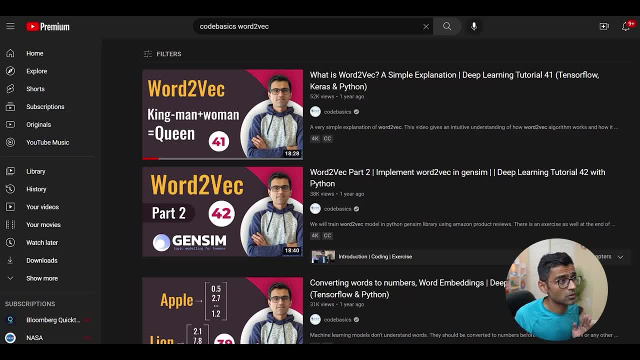 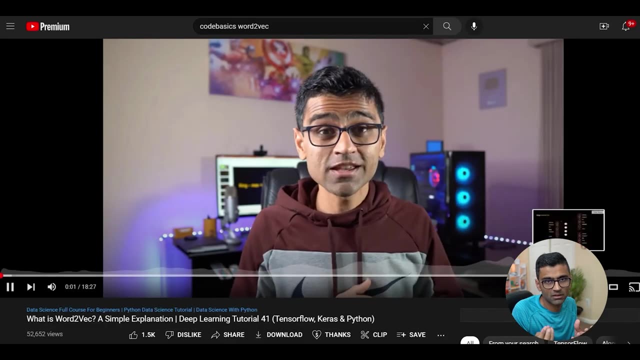 made a different video. so if you go to youtube search for code basics, word2vec- that that first video that you see, which is part of my deep learning playlist. please watch that because that will give you a very good understanding of the actual method or actual technique behind word2vec. since i already have that video, i'm not going to repeat the same. 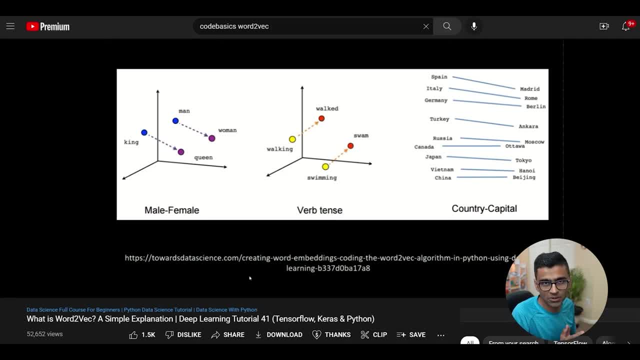 thing, so i'm not going to repeat the same thing. so i'm not going to repeat the same thing here. i would highly recommend you watch that. okay, if you don't watch it, you're going to probably miss few things in this nlp series. so word2vec- very, very important concept- you need to watch. 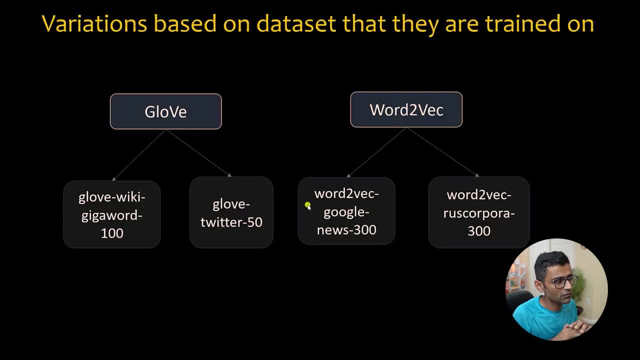 that video. now there are variations based on the data set that they are trained on. for example, word2vec, you can train on google news data set or some different corporates and based on that you can get different variations. so word2vec is like a technique, but you can use that technique on different data set. it's like you are training. 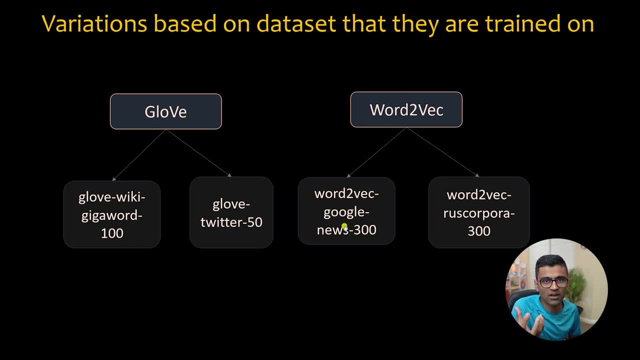 support vector machine. so support vector machine is one technique, but you can train it on amazon reviews or movie classification. similarly, word2vec, the actual embedding vector, you can get by training it in a different corpus, same like glow. if you train it on twitter, let's say there is a glow twitter 50, this model, which is available in gensim live. 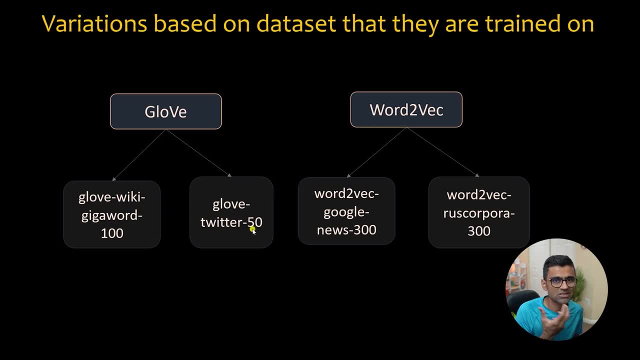 library. it will understand the tweets better, all the slang and all the short form that you use. it will understand that better. and then there could be a wiki giga word glow version. there are so many different models, but the basic techniques are glow, word2vec, fast text and so on. similarly, 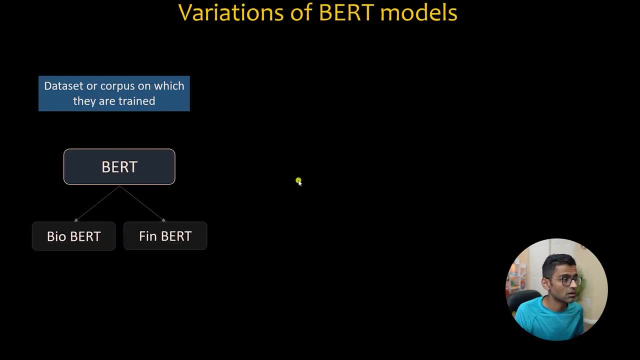 the transformer based models such as bird, also based on what type of data set they're trained on. you can get bio bird or fin bird. fin bird is trained on financial data set. bio bird is trained on biomedical database and you can also do some parameter tuning in bird and get things like albert or roberta. 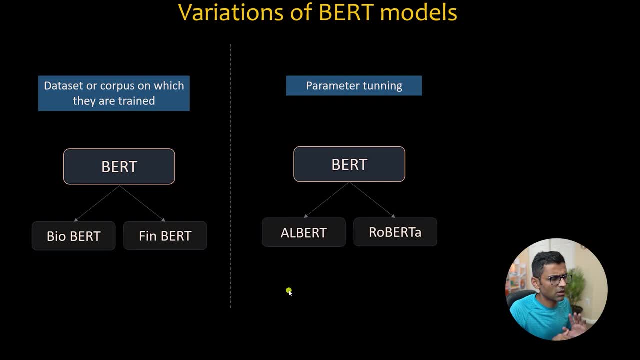 so you would hear all these jargons. you know finbert, albert, roberta, word2vec, so i'm just throwing all the jargon so that you get some overview. don't worry, if you don't understand these techniques, we'll go over them in detail. 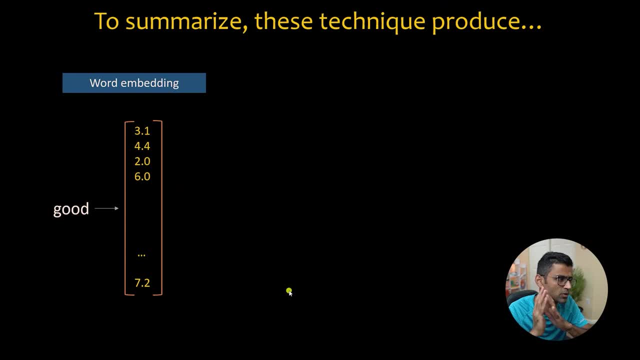 in the later video. but just to summarize what these techniques produces: see, folks, it's very simple. the whole purpose of these techniques is to convert word into a vector, because, we have seen previously, machine learning models don't understand text. they need numbers. so you can convert a single. 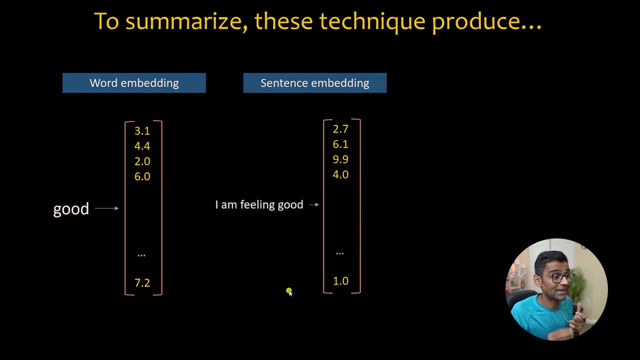 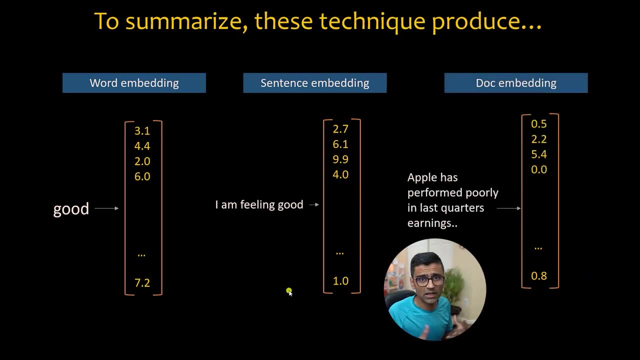 word such as good to a vector. you can convert entire sentence to a vector, and that is called sentence embedding. or you can convert a single word to a vector, and that is called sentence embedding. or you can convert the entire paragraph or a news article or a document into a vector. so in